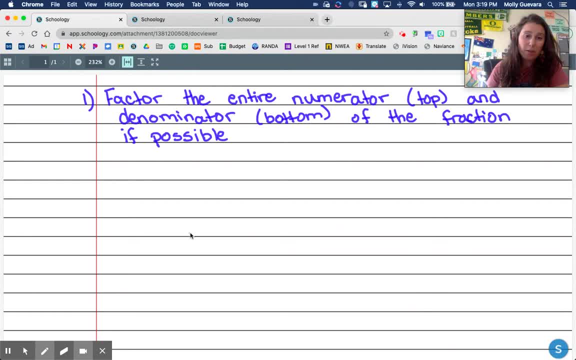 top of the fraction, or we're not able to factor the bottom of the fraction, and that's okay too. Okay, let's look at our second step, and I'm going to go ahead and type it in here. So we're going to type it in here and write it in, and then we'll go over it. 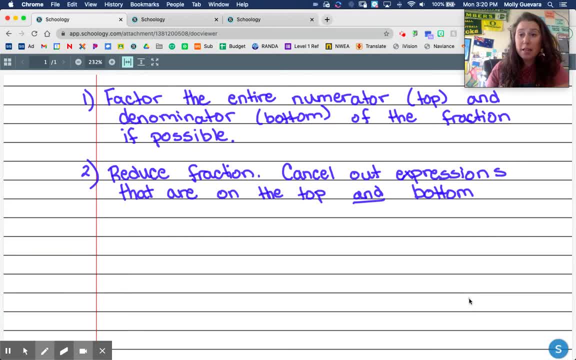 All right. so here's the second step. You want to reduce that fraction, meaning anything that's on the top and on the bottom, both. so in the numerator and the denominator you can cancel those out, So any common terms that are both on the top and the bottom. 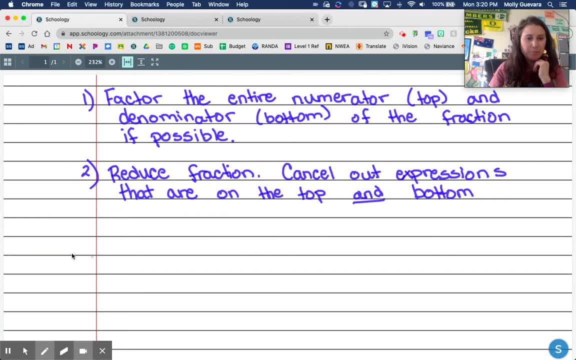 you can go ahead and cancel out, and that will help reduce your fraction. Okay, our third step here is to rewrite the remaining expressions. So whatever is left, okay, so, after you've crossed things out, what is left on the top, What is left on the bottom? So that's what you're going to want. 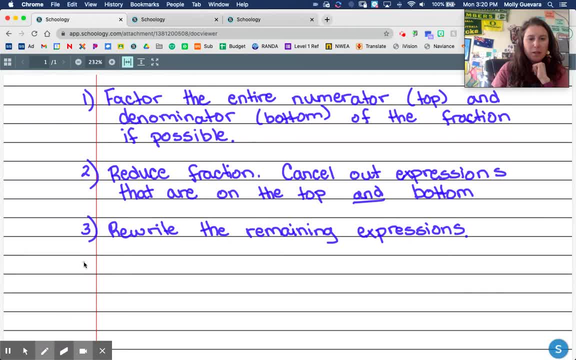 to do in step three. Okay, and then the last step, step four. again, I'm going to write this down and then we're going to talk about it here for in a second. Okay, so here's the fourth step. So step three is to state any values that would make the denominator zero. So remember, 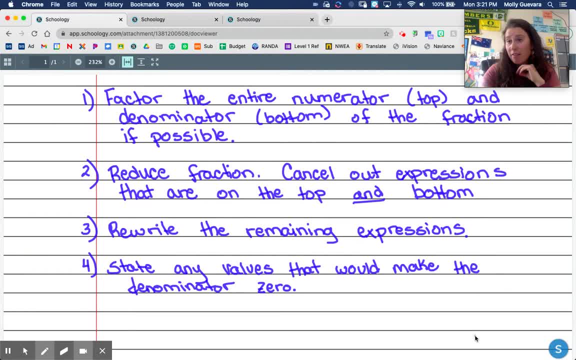 the one rule that we have with fractions is that I can never, ever, ever have zero on the bottom of a fraction, So I have to include what values on the bottom I would not be allowed to plug in. So if I have a variable, let's say x, right in the equation, in the expression: 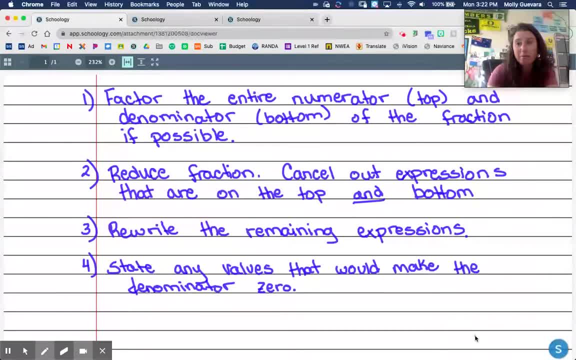 what values would I not be able to plug in for x? zero on the bottom. So let's look at – it looks like we have three examples here. So let's look at a couple examples on just how do we simplify these rational expressions. 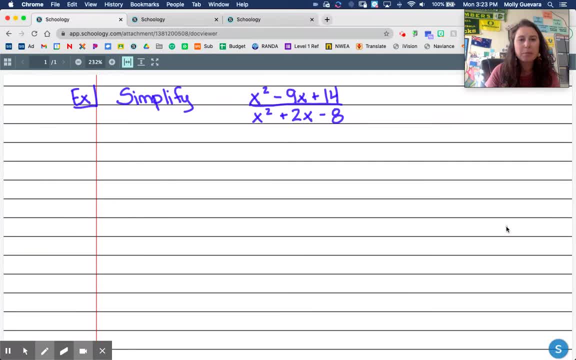 Here's our first example for today. It says: simplify X squared minus 9X plus 14 over X squared plus 2X minus 8.. So step one that we just wrote up above says to factor the entire numerator and denominator if possible. 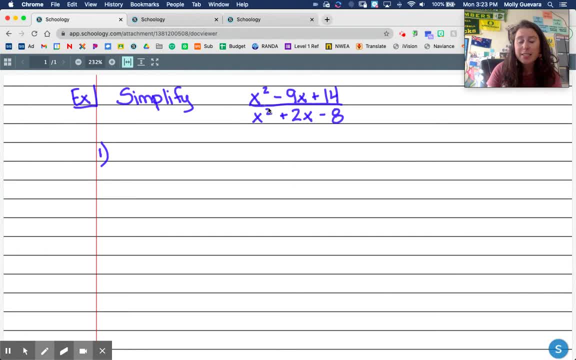 So I need to look at the – let's just start with the numerator and see if this is factorable. So here I have a trinomial quadratic: A is 1, right, the number in front of X squared is 1.. 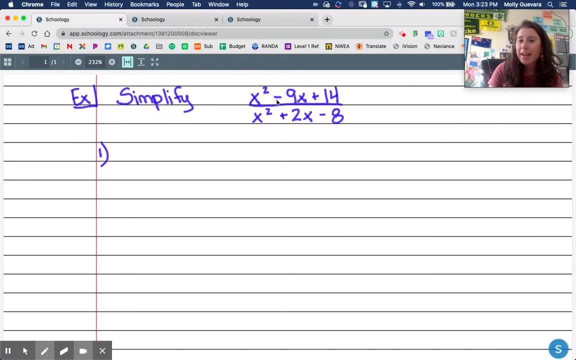 So I'm looking for what are two numbers that multiply to 14 and add to negative 9.. So if we go down the list right, 14 and 1,, 7 and 2 actually ends up working for us here, as long as they are both negative. 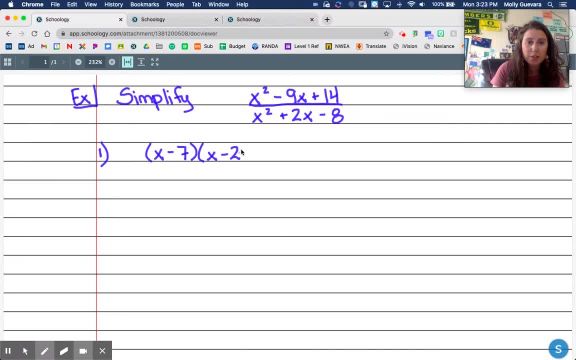 So X minus 7.. X minus 2 is the top factor And then the bottom. here I have X squared plus 2X minus 8.. Again, it's a trinomial, It's a quadratic And A is 1.. 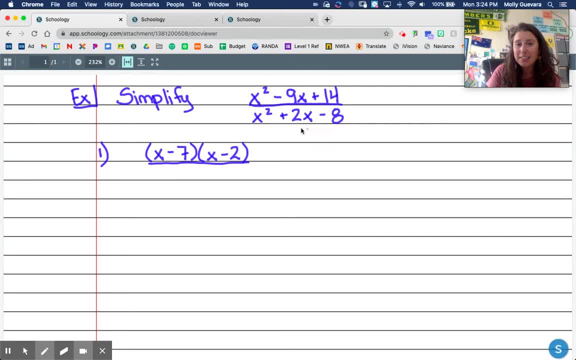 So I'm looking for two numbers that multiply to negative 8 and add to 2. So that is going to give me positive 4 and negative 2.. X minus 2.. X minus 2.. X plus 4.. Okay now step two says to reduce the fraction. 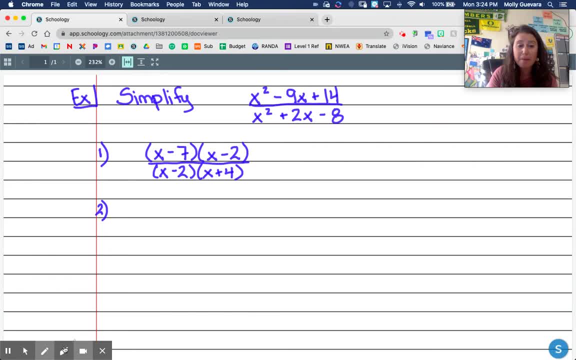 So I'm going to cancel out anything that's common on both the top and the bottom. So here on the top I have an X minus 2 and on the bottom I have an X minus 2.. So those can cancel. We're going to make a note here that we can cancel the X minus 2.. 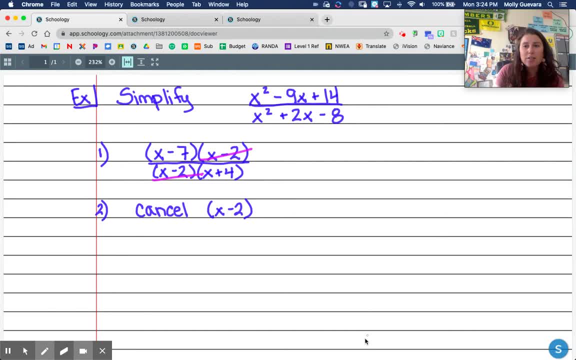 I cannot cancel the X minus 2.. I cannot cancel the X minus 2.. I cannot cancel the X out of the X minus 7 and the X from the X plus 4.. These are locked in with the parentheses, and so I'm not able to simplify those at all. 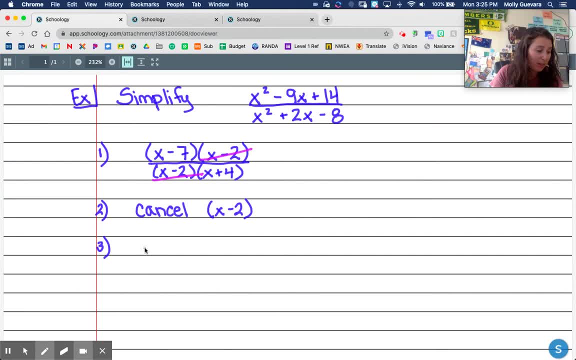 Step three says to rewrite what's left. So what's left is X minus 7 on top. Since there's only one parentheses, you don't have to write the parentheses And X plus 4 on the bottom. Okay, And the last thing is I have to figure out any values that would make the bottom zero. 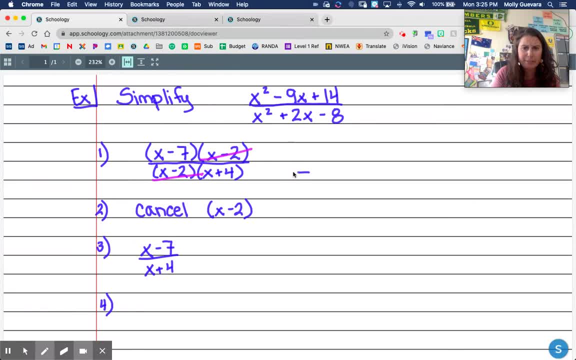 So I'm going to look right here on the bottom, Right here, In order for the bottom to be zero, I would have to figure out what X would be in this parenthesis and what X would be in this parenthesis to get zero. So I'm going to take each term with an X in it. 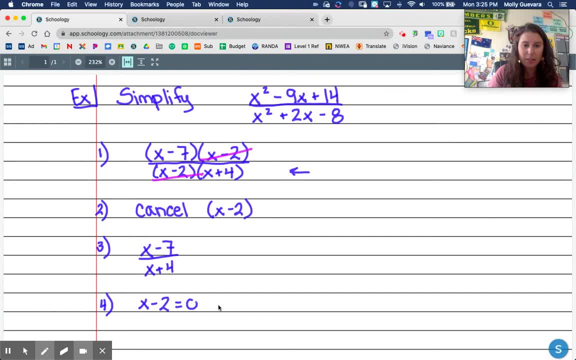 So X minus 2 is one of them, and I'm going to set it equal to zero. And then X plus 4.. X plus 4 is the other one. I'm going to set it equal to zero And I'm going to solve. 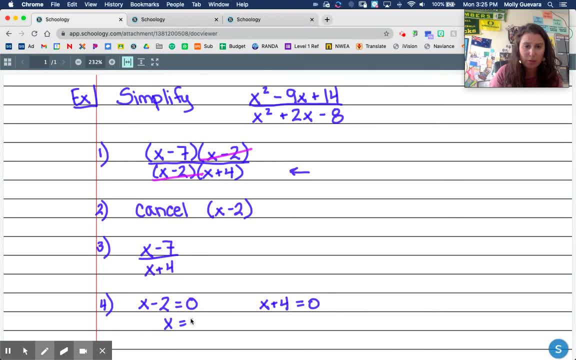 Right, So I get X equals 2 and X equals negative 4.. So those are the two values that X is not allowed to be, Because if I plug in 2, I have 2 minus 2, which is zero, and zero times. whatever this is, which. 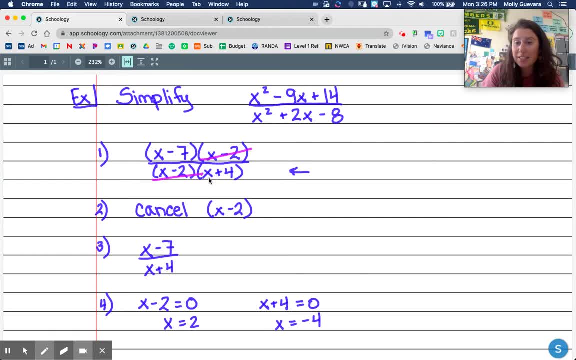 would be 6.. Right, Zero times 6 is zero and I get zero on the bottom of the fraction, which I can't have Right. So if I plug in negative 4, I have negative 4 plus 4, which is zero, and it will be negative. 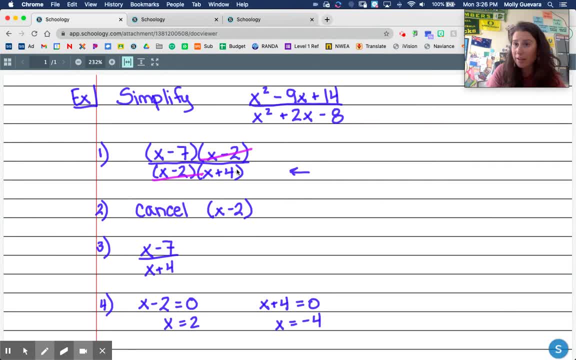 6 over here And zero times negative. 6 is zero, and you can't have zero on the bottom, So that's why these values are coming in. So my final answer, after simplifying, is X minus 7 over X plus 4. and then we also have to write: 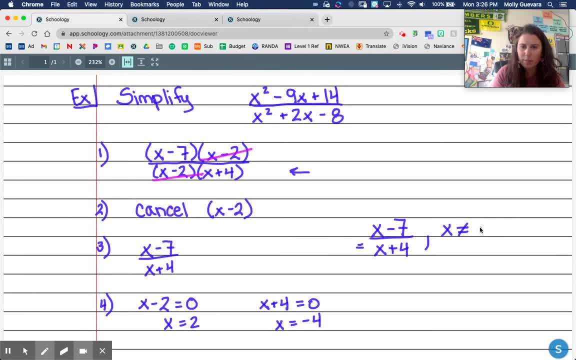 that X cannot be negative, 4 or 2.. Right, So those are the two values that I am not allowed to have for X. Other than that, I can plug in anything I want: Negatives, positives, zero. Anything I want, except for negative 4 or 2.. 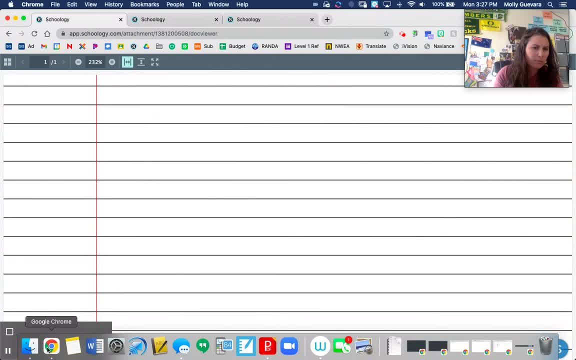 Let's look at another one now. So our second example says to simplify, Okay, Simplify 2 minus X over X squared minus 4.. Okay, So, first step factor: There's nothing to factor on the top, since that is linear. 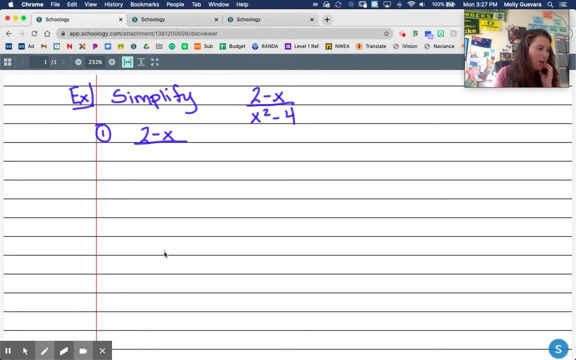 Right, That's just a line, Nothing to factor On the bottom. I have a perfect square minus a perfect square, So we can use the difference, The difference of squares. So the square root of X squared is X. The square root of 4 is 2.. 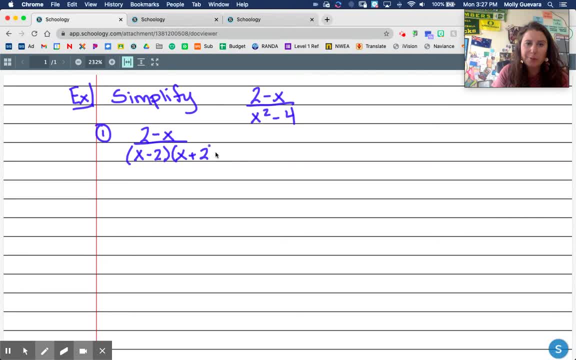 So I have X minus 2, X plus 2.. Now if we notice, nothing cancels Right Here this kind of looks the same: 2 minus X and X minus 2.. But let's notice, here the 2 is positive. 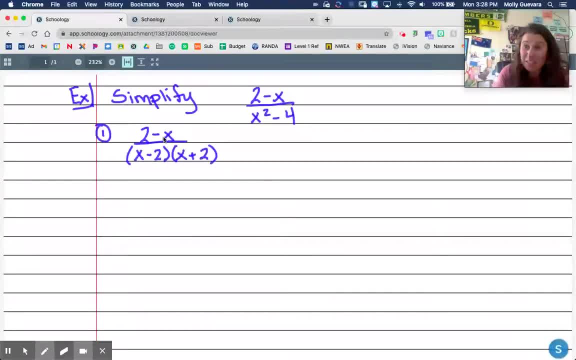 Here the 2 is negative, Here the X is negative, But both of these the X is positive. So I'm not really sure if anything cancels. So the thing to try, if this ever happens, is I'm going to take out a negative 1.. 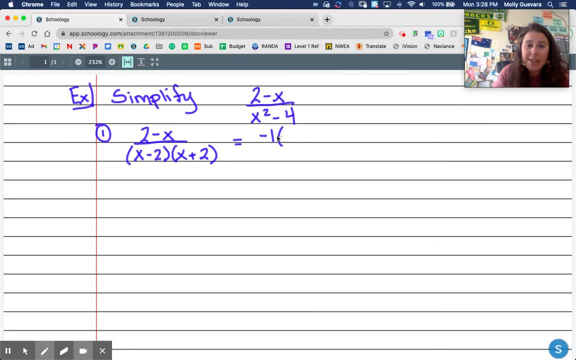 Because I can do that. that's okay. If I take out a negative 1, this positive 2 becomes negative 2. And this negative X becomes positive X, And I still have X minus 2 on bottom and X plus 2 on bottom. 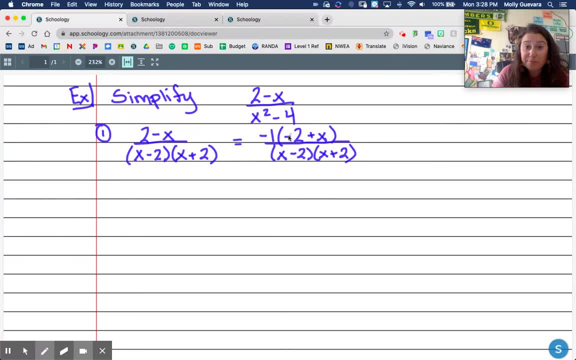 Okay, Now let's look Now. my 2 is negative and my X is positive. So now I am able to cancel with this first parenthesis, where my 2 is negative and my X is positive. Right, So I can. now I can cancel these two out. 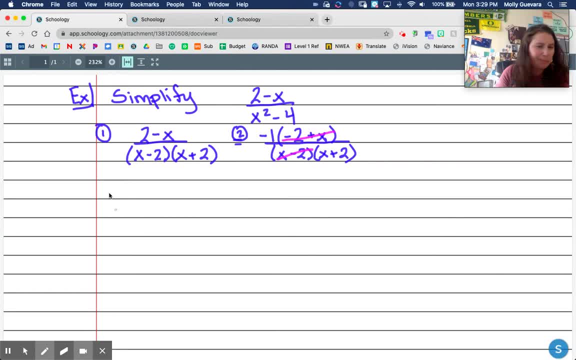 That's kind of my step 2 there. right is canceling. Step 3 is to write what's left. Well, what's left on the top is negative 1, because everything else canceled, And what's left on the bottom is X plus 2.. 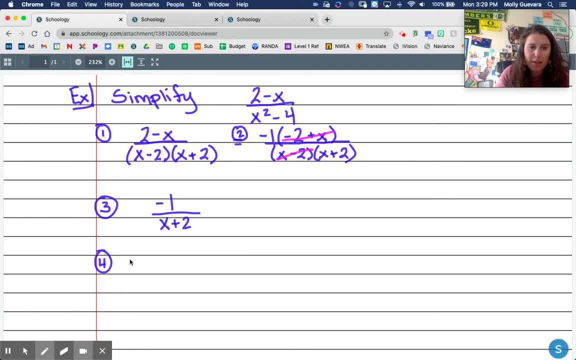 That's okay. Then the last step is: I have to figure out what I'm not allowed to have. So I'm going to take my factored form, which is X minus 2, and I set it equal to 0.. And then my other parenthesis, which is X plus 2,, set it equal to 0.. 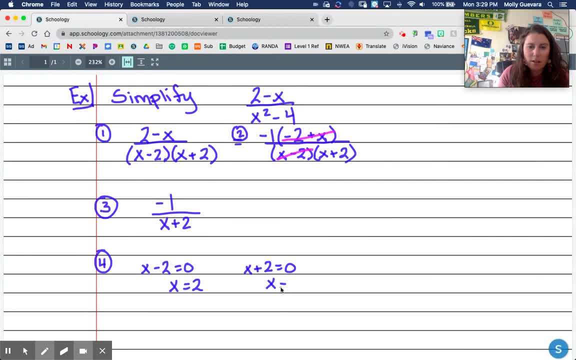 So I get X equals 2 and X equals negative 2.. So those are the values I'm not allowed to have. So my final answer is 1 over X plus 2, but X cannot equal negative 2 or positive 2, because 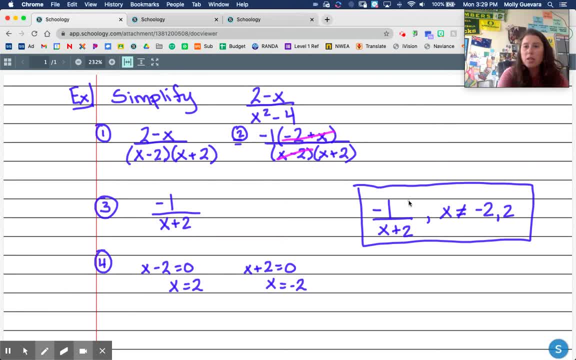 if I enter a negative 2 or a positive 2, I will get 0 on the bottom of our fraction, which I'm not allowed to have. All right, Let's look at one more and then we'll be cruising, Okay. 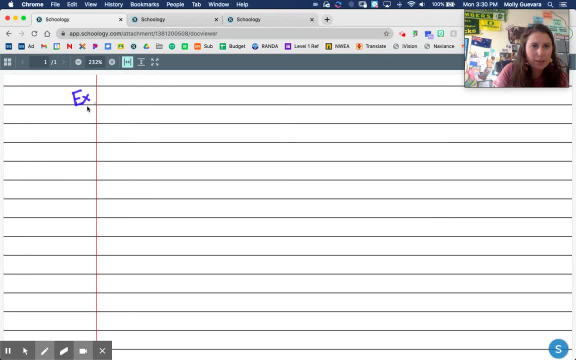 All right, Okay, Last one. I want to simplify: X cubed plus 4X squared minus 9X minus 36, over 4X squared plus 28X minus 36.. Okay, X plus 48.. Holy moly, that escalated quickly. 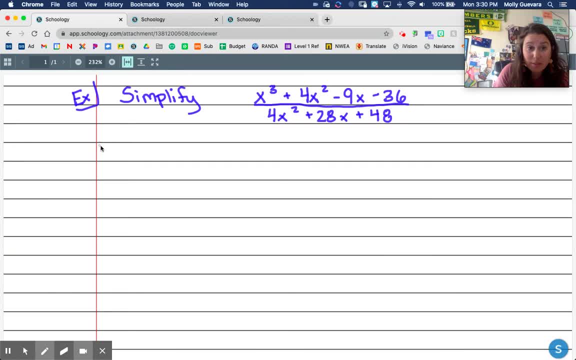 Right. Step one is that I have to factor. That's my first step. Now I'm going to stay very, very, very organized here. I'm going to focus on factoring the top first. Okay, So I'm just going to rewrite the numerator, like so. 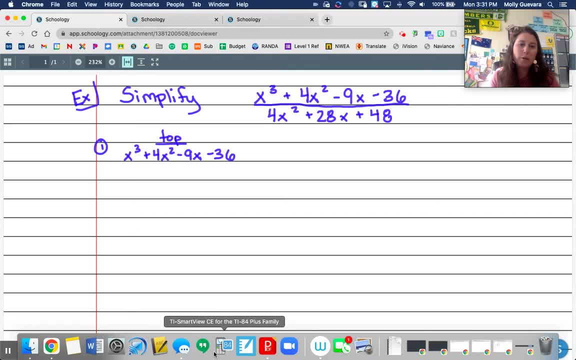 Now, with this numerator, I have four terms And anytime you have four terms, factoring by grouping should be your first thought. If I group these first two terms together, my greatest common factor is an X squared. If I take out an X squared, I'm left with X and I'm left with 4.. 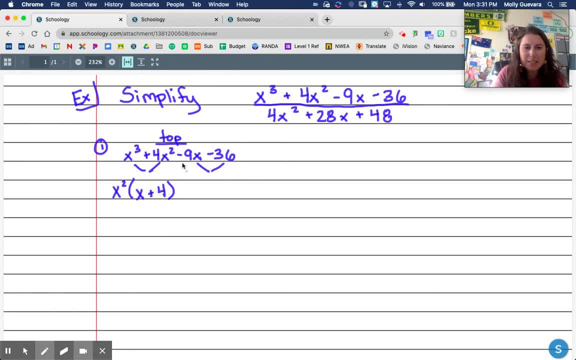 Okay, My second. If I group my This set of last two terms together, I have a negative 9X and negative 36.. My greatest common factor here is negative 9, which leaves me X And negative 36. divided by negative 9 is positive 4.. 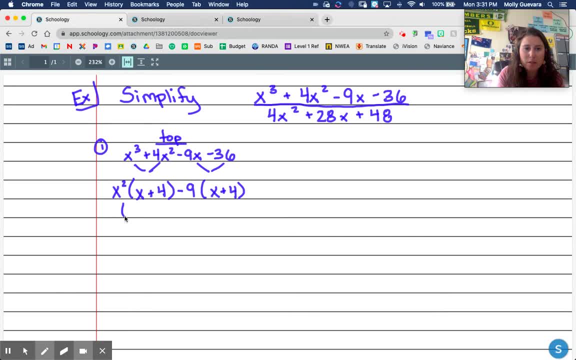 Remember, you always want your parentheses to be the same, So that gets me X plus 4, just one of them, And then my two terms outside the parentheses, so X squared and minus 9.. And my remaining terms, However: X squared minus 9, is a perfect square. 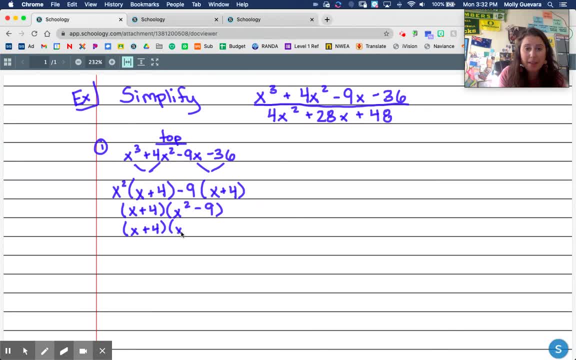 So that is actually factorable again And that gets me X plus 3 or X minus 3.. Remember, you can do the minus 3 first, It doesn't matter. So that is the top of my rational expression factored. 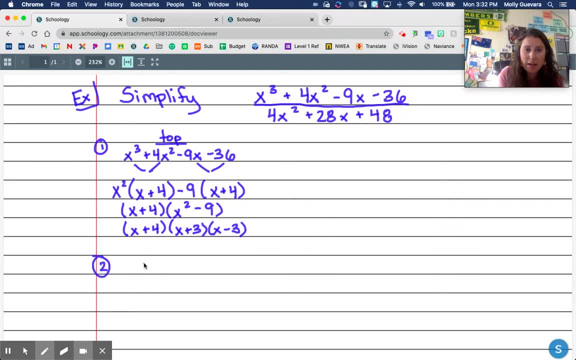 So for step two, when we're going to go ahead and simplify, I'll just go ahead and write this out. So the numerator, The numerator is X plus 4, X plus 3, X minus 3.. Now let's look at the bottom. 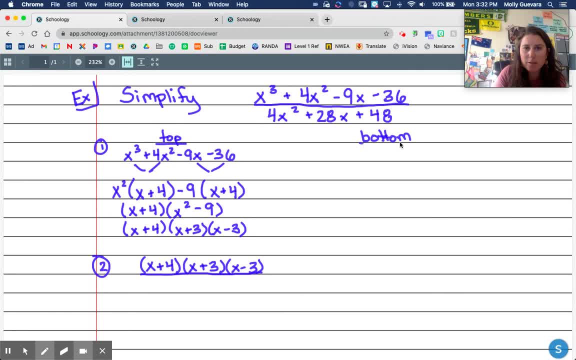 Right, Because I have to factor the top and bottom if possible. So here I have 4X squared plus 28X plus 48.. You should always check for a greatest common factor first, And in this case I do have a greater. 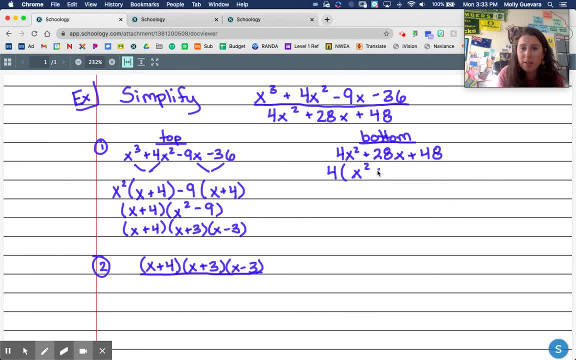 This is the greatest common factor: It's 4.. So that leaves me X squared plus 7X plus 12.. And what's nice about that is that I now have a quadratic, a trinomial, where A is 1.. 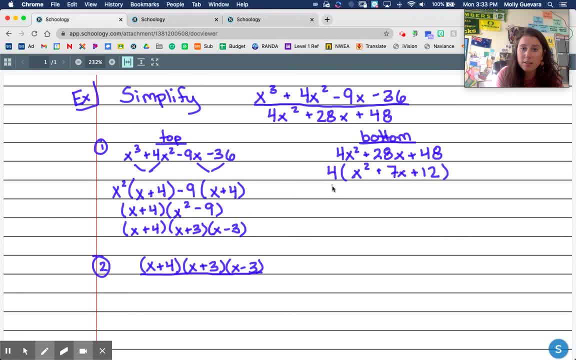 So I'm able to factor this pretty quickly in our heads And so hopefully we see the two numbers that multiply to 12 and add to 7 is X plus 5.. Oh gosh, X plus 3.. That's what I get for looking ahead. 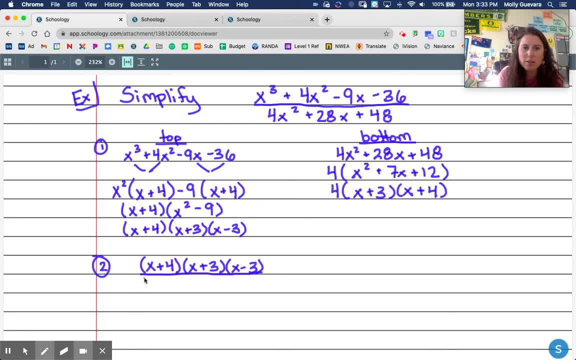 And X plus 4.. Okay, So there's the numerator factored And so I can go ahead and write that down. Okay, So I have factored the top and I have factored the bottom. That is step one. 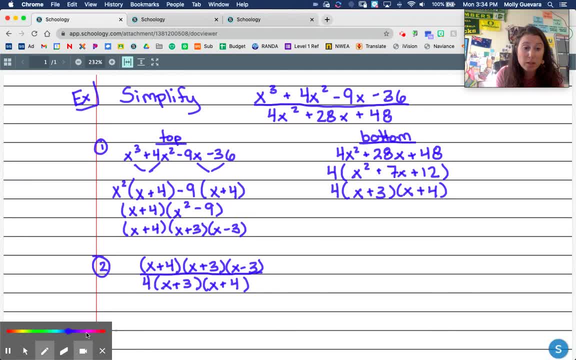 Step two: I want to cancel anything that's common on both the top and the bottom. So when we look here, I have an X plus 4 on top And on bottom. I also have an X plus 3 on top and on bottom. 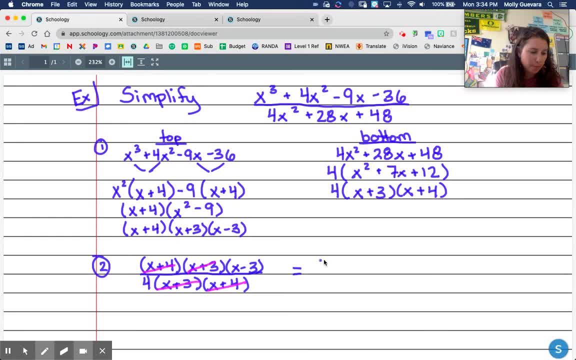 So that leaves me right in step three to rewrite it. What's left on top is an X minus 3.. And what's left on bottom is a 4.. And then the last thing is, I just have to figure out what values I'm not allowed to have. 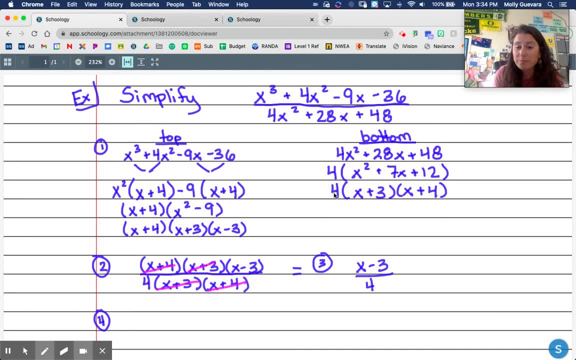 So when I look at the bottom, 4 doesn't have a variable with it. It doesn't have an X, So I don't have to set the 4 equal to 0. It's only terms with a variable in it. 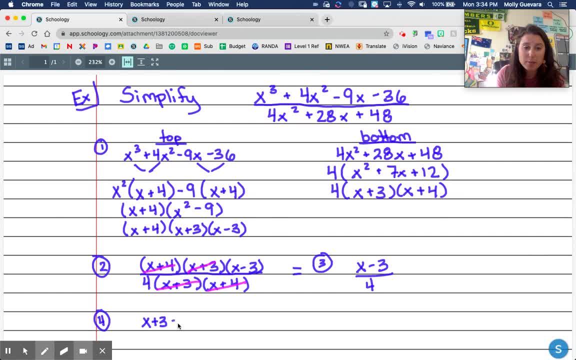 Okay, But I do have to set my X plus 3 equal to 0,, which gets me negative 3.. And I do have to set my X plus 4 equal to 0,, which gets me negative 4.. So those are the two values that X is not allowed to be.